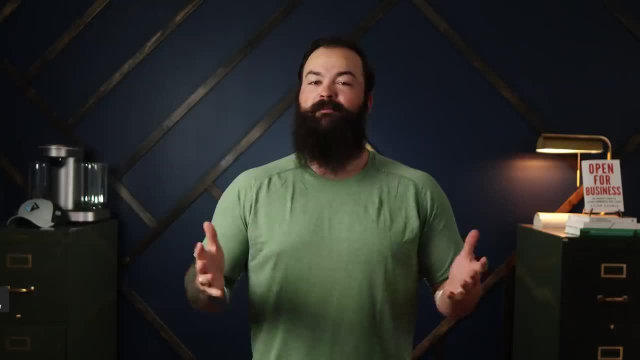 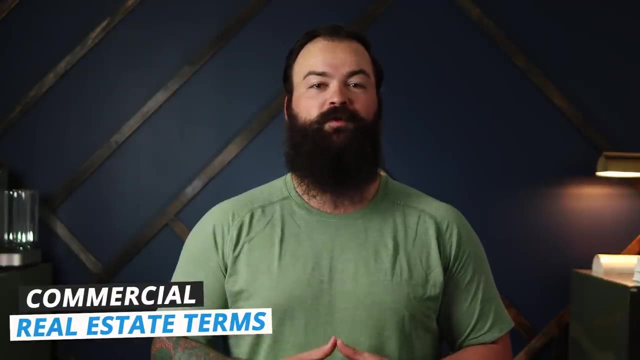 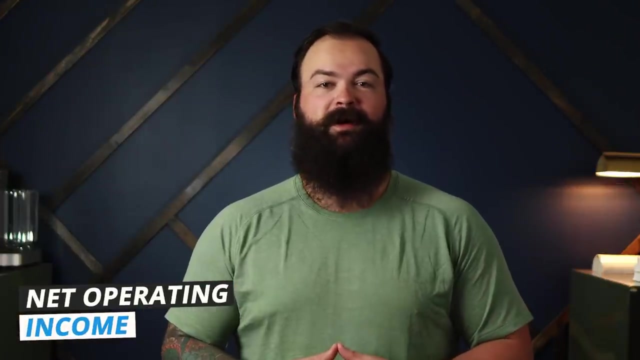 started so that you don't miss any important information. Let's dive on in Up. first are general commercial real estate terms. The following terms and calculations are some of the most commonly used in commercial real estate dealings: Net Operating Income: You may be familiar with this term from your residential investing experience. 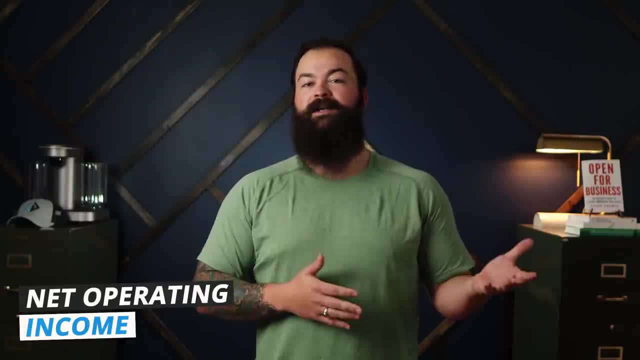 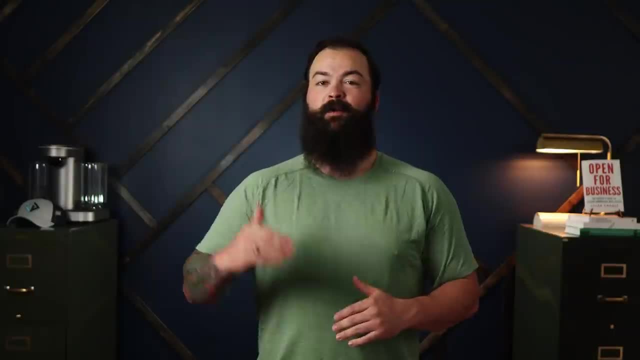 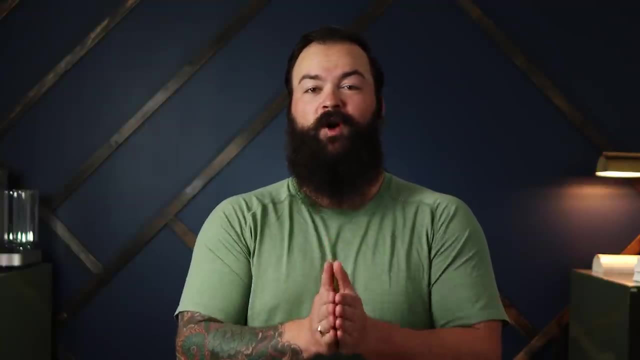 NOI is equal to your gross rental income minus your operating expenses. Note that these expenses do not include any mortgage payments or depreciation. As your NOI increases, property value also increases, and vice versa. NOI is an important term to know as it determines your current. 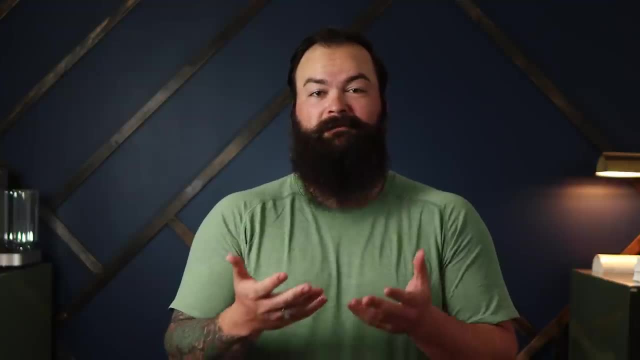 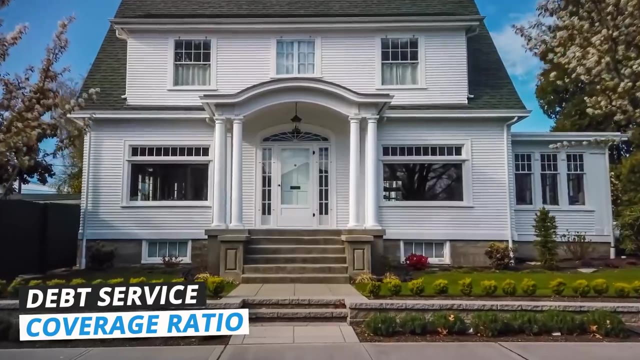 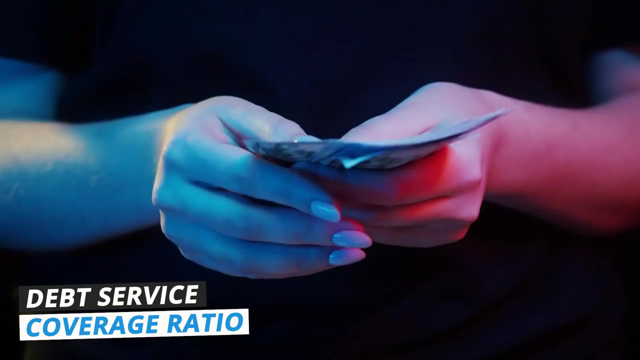 and future property value, how you make an offer and any future potential cash flow. Debt Service Coverage Ratio. The Debt Service Coverage Ratio, or DSCR, is a term used often when dealing with lenders and financing. DSCR is equal to your NOI divided by your annual debt. The Debt Service Coverage Ratio can determine: 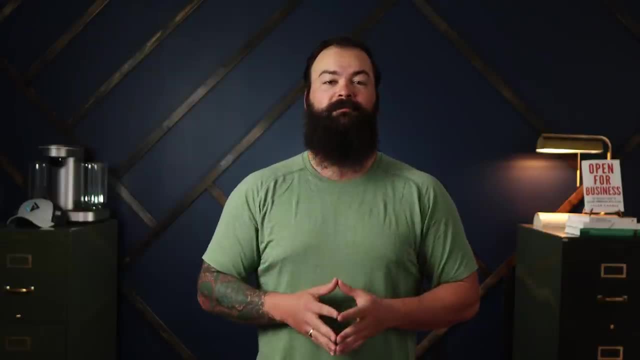 the amount of cash flow you have to pay your mortgage and hopefully make a profit. Commercial lenders want you to be able to pay the mortgage and have plenty of room for something left after. This is an important number that lenders check first to see if a deal is lendable. and is the first number that we check when underwriting a commercial real estate investment. Let's explain this calculation a bit more. The Debt Service Coverage Ratio equals your NOI divided by your annual debt. If it calculates to 1.0 or less, then you have no excess cash flow. Essentially, your NOI is equal or less than your mortgage. If it is higher than 1.0, that means the property should have cash flow. Lenders typically look for a Debt Service Coverage Ratio of at least 1.2, if not 1.25 or more. 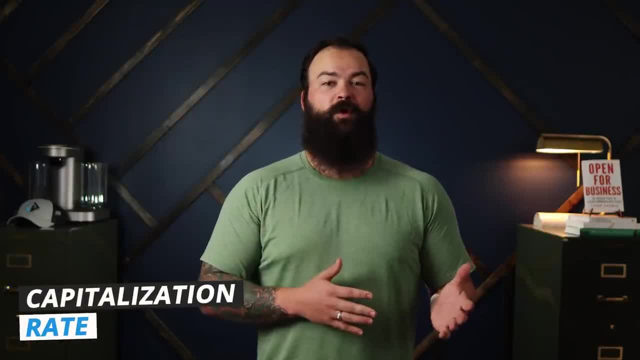 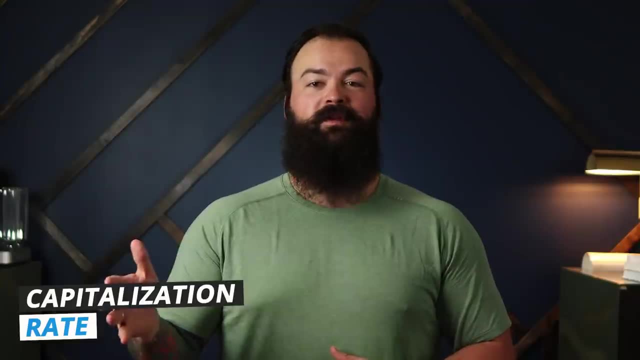 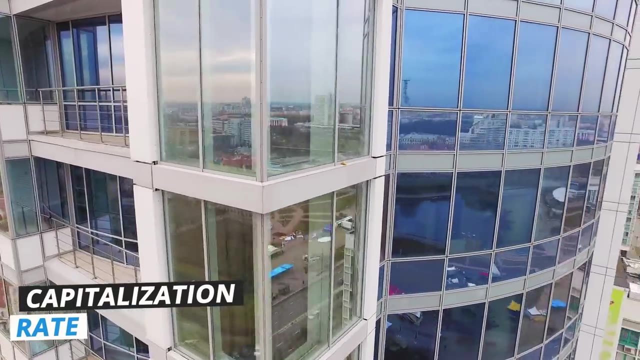 Capitalization Rate. Capitalization rate, or cap rate for short, is a calculation used by just about every single investor in the commercial real estate industry. Cap rate is equal to the NOI divided by the sales price. Cap rate is used to measure a building's performance without considering the financing. 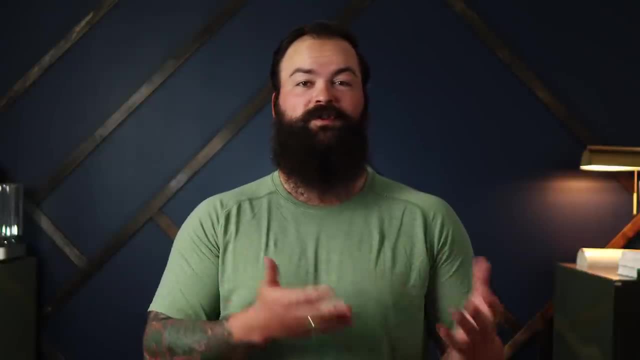 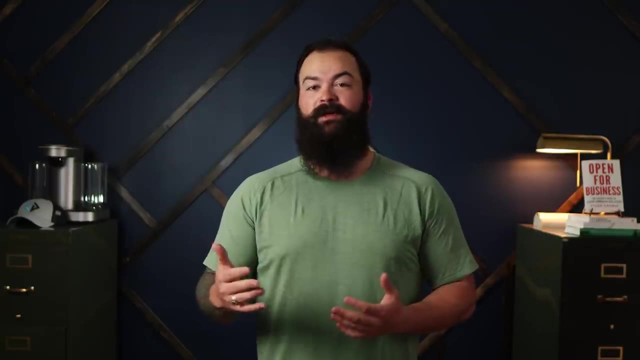 on the building. Thus, a cap rate is essentially equal to your return on an investment if you paid all cash for the property. Cap rates can vary significantly depending on the age of the building, location, property type, lease terms and more. Now let's talk about high and low cap rates. for a second. A high cap rate, such as 10 or 12%, usually signifies a high cap rate. A high cap rate signifies a high risk investment with a lower sales price. High cap rate investments are usually located in lower income neighborhoods. have higher vacancy, lower future potential or just require more work. A low cap rate, such as 4-6%, typically indicates a lower risk investment with a higher sales price. Low cap rates are usually found in upper middle class or upper class neighborhoods. 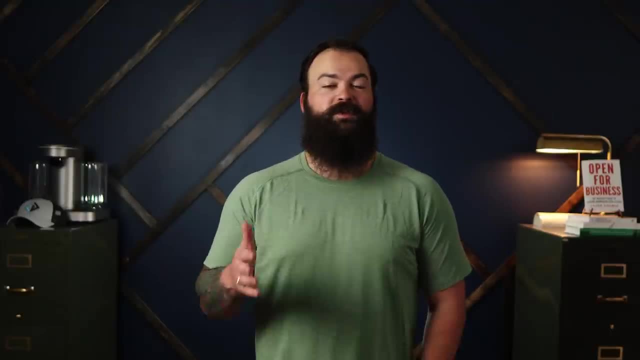 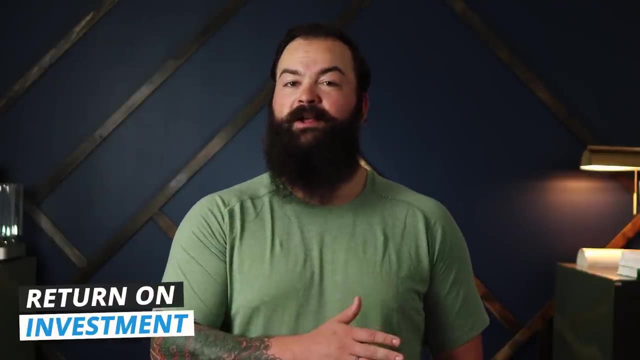 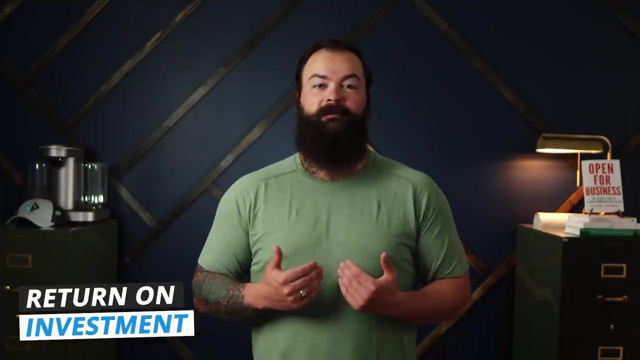 and come with national credit tenants and longer term leases. Return on Investment: Return on investment is basically your annual cash flow divided by your down payment. ROI is measuring how fast your money is coming back out of the property, which is very important for you to know as an investor. 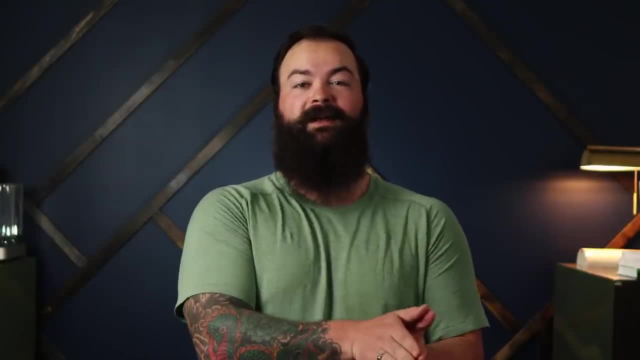 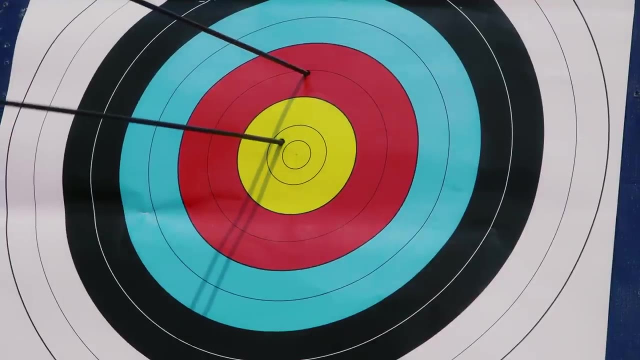 After all, you want to know how soon you will make your money back and be able to compare different investment opportunities. I think it's very important that you set an ROI target and stick to it. I won't invest in a deal where I won't get at least a 15% cash flow. 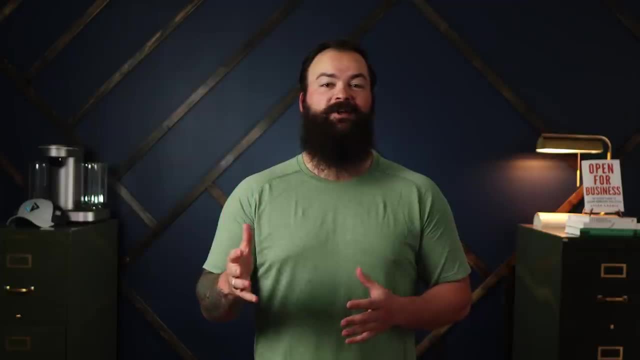 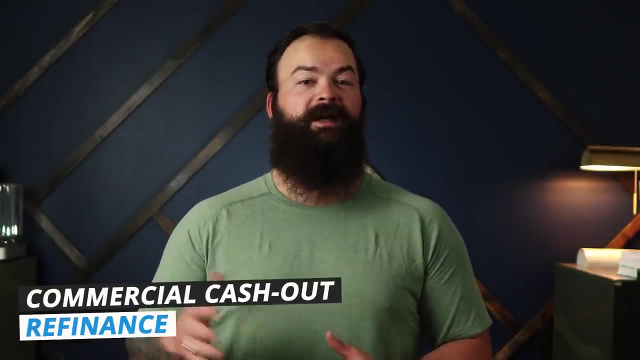 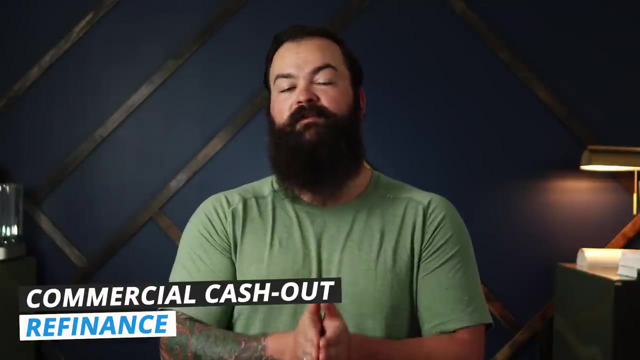 cash-on-cash return on my investment. Every deal you do could take cash and time away from another opportunity. Commercial Cash-Out Refinance: A commercial cash-out refinance is basically buying a commercial property, then increasing the net operating income through rent increases and expense reductions and finally refinancing. 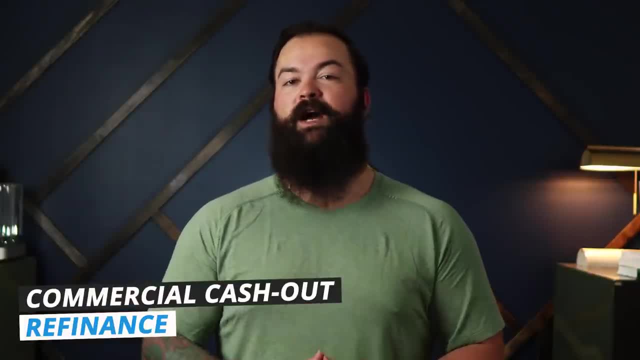 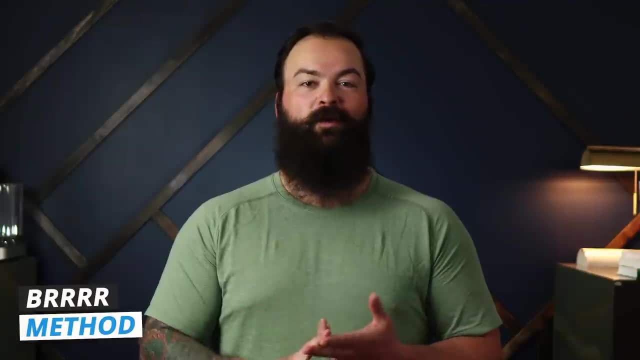 the loan to pull out the original down payment or your investor's down payment while maintaining ownership of the property. You likely know this more commonly as the BRRRR method- Buy, rehab, rent, refinance and repeat- made famous here at BiggerPockets by Brandon Turner. 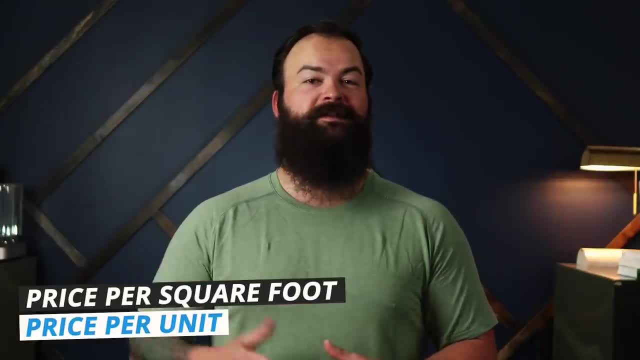 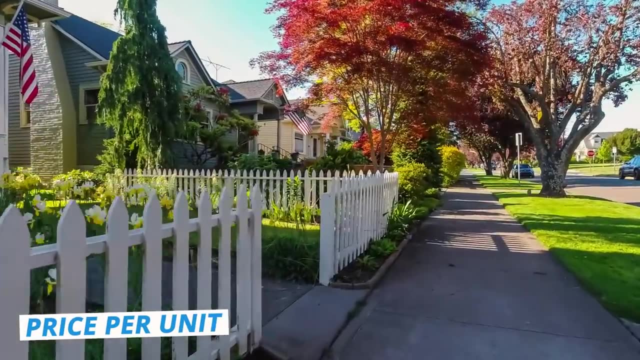 Price per square foot and price per unit. You may have heard these next terms before if you have a background in real estate. Price per unit: This calculation helps buyers and sellers determine a property's value. It varies depending on the neighborhood or what sub-market in which the property is located. Price per unit is a calculation usually used for apartments and is calculated by dividing the price of the property by the number of units. If you have a million-dollar apartment, you can divide the price of the property by the number of units. If you have an apartment building and you have 10 units in it, that's $100,000 per unit. Comparing your price per unit in your market with your property's price per unit can give you a quick snapshot of the potential of a deal and help you ensure your offer price and the seller's asking price are both within reason. Price per square foot. To determine the price per square foot, you use the same calculation as price per unit. 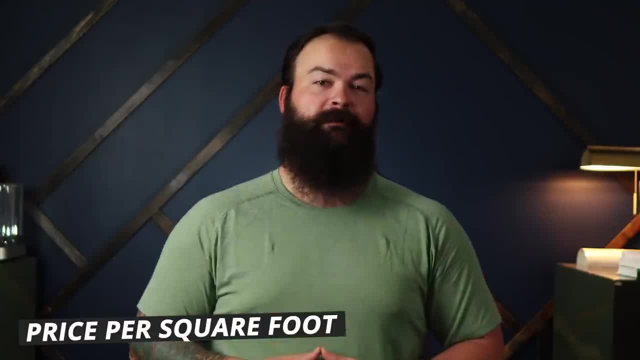 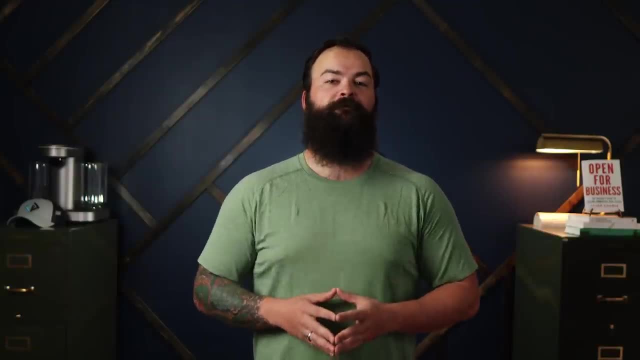 but instead you divide that price by the square footage of the building. So let's say the building is a million dollars and it's 10,000 square feet. that would be $100 per square foot. We use this calculation for offices, retail centers and industrial buildings. 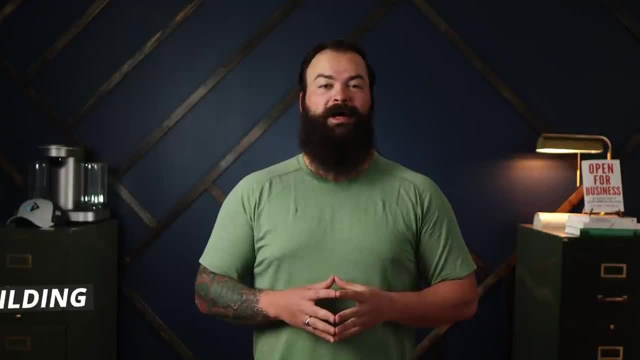 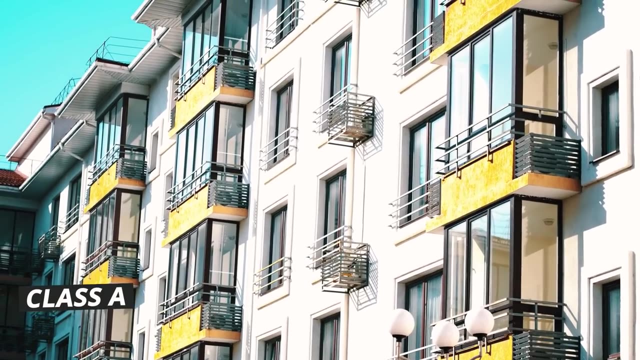 and it's actually the method that I use to buy my first building. Building Classification: Commercial buildings are separated into three separate classes based on their characteristics: Class A Buildings: Class A buildings are the newest and highest quality, with the best location and highest rents. They're in great neighborhoods and attract top-tier tenants, So they're typically downtown and may have commercial on the main level, with office hotels or residential units on top. Class A buildings are not typically for new investors, since prices are high and the market is competitive. 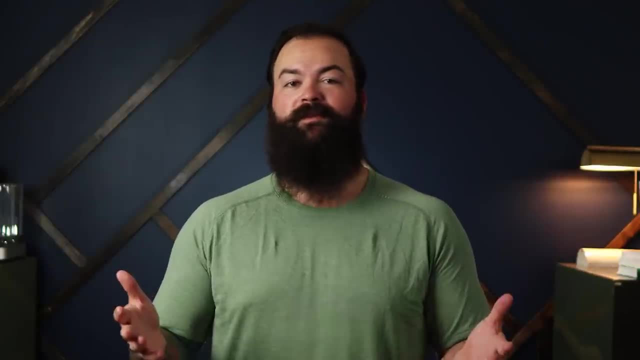 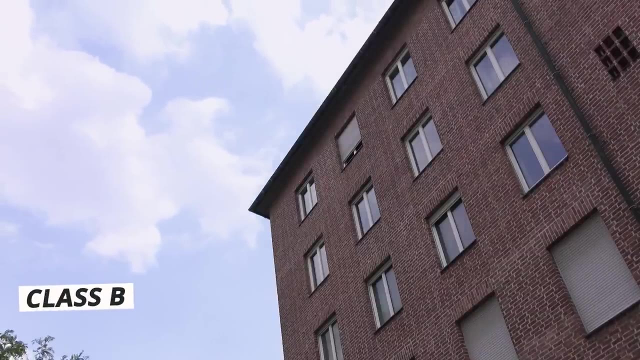 Seasoned buyers and funds can pay all cash and they're just fine with the lower returns that these properties bring. Class B Buildings: Class B buildings are often older than Class A buildings, but they are still good quality and attract average to above-average tenants. 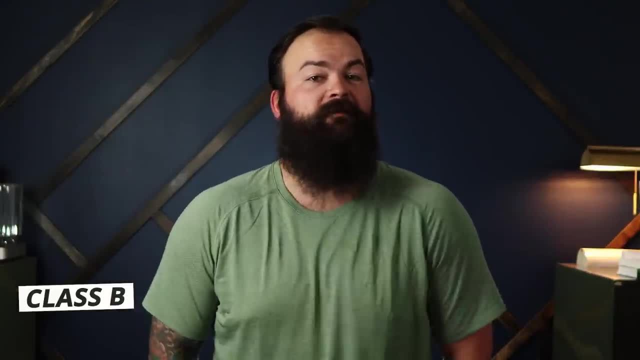 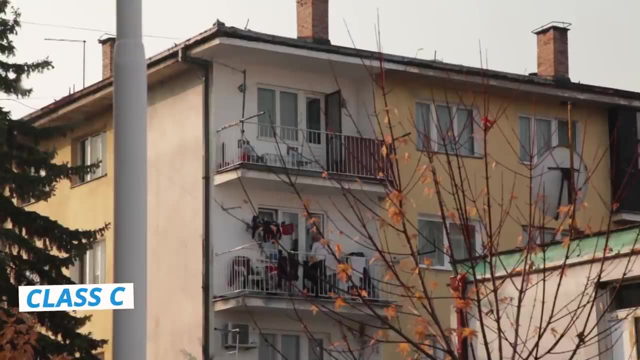 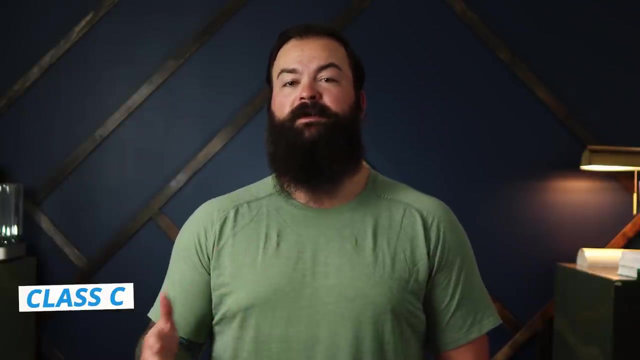 They're relatively stable properties that are oftentimes targeted by value-add investors, since there is room to make improvements and raise rents. Class C Buildings: Class C is the lowest official classification and the buildings are older and likely in need of renovations. They have the lowest rents and usually low- to mid-tier tenants. Apartment investors often target Class C buildings because the ratio between the price per unit and the rents are still good and can allow for some of the highest returns. There will always be demand for these buildings, since more properties are becoming Class C every day, but this building stock does require a lot of rents. 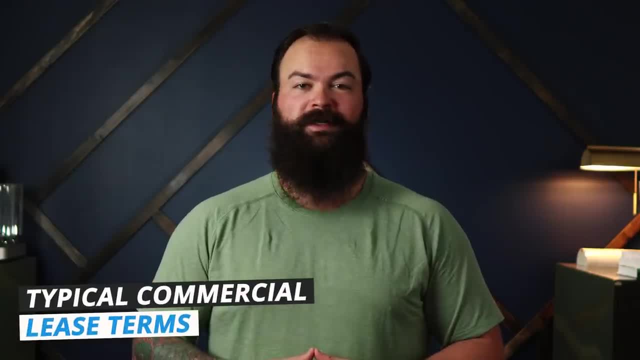 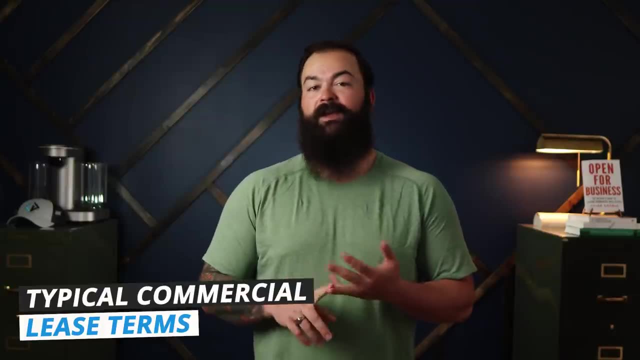 The price per unit is a lot of maintenance and management skills. Now let's cover typical commercial lease terms. Commercial leases can be structured in a variety of ways depending on the type of property, type of business and the number of tenants. Here are a few of the most common structures that you'll see. Triple Net. A triple net lease or a net lease is one of the most common lease structures. It requires the tenant to pay base rent along with the three nets: Property taxes, building insurance and common area maintenance, or CAM for short. With triple net leases, the tenant incurs all expenses related to the property, but the landlord is not off the hook. They are still responsible for maintaining the structural components, such as the structural walls, foundation and roof of the building, The only time the landlord is completely free. of responsibilities is when the tenant has an absolute triple net lease, where the tenant is responsible for the structural components of the building as well. To calculate rent for a triple net lease, you take the estimated annual expenses and add that number to the price per square foot. 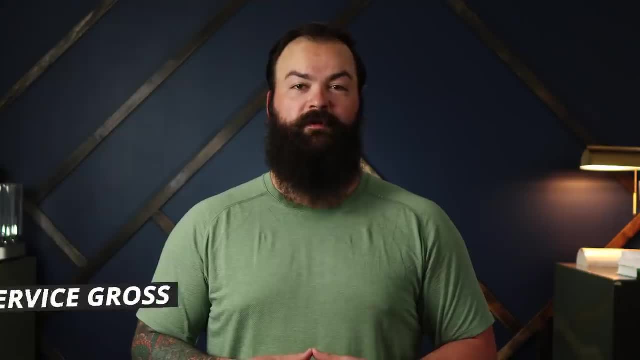 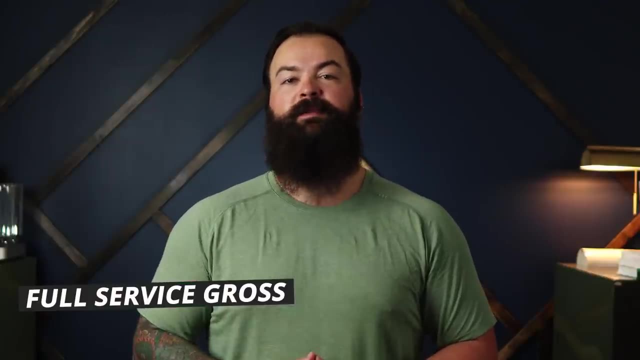 multiplied by the amount of rent that the tenant is responsible for: A full-service gross or FSG. A full-service gross lease, or sometimes referred to as a full-service lease, requires the tenant to pay a base rent, while the landlord incurs all expenses related to the 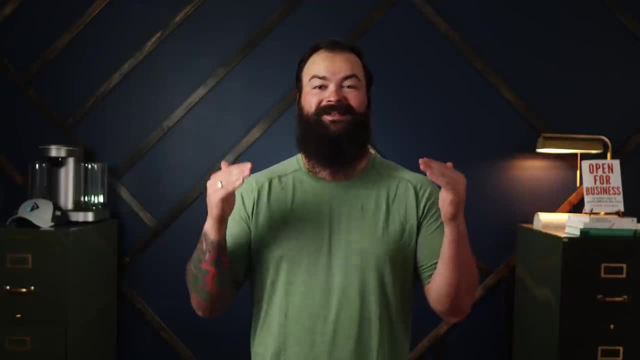 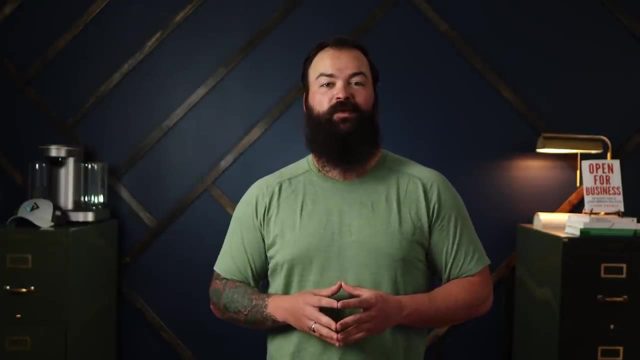 property. This lease structure can be great, considering that the tenant knows exactly what they are paying each month, but it can also be a double-edged sword. The property owner will probably significantly increase the base rent of the space with a full-service gross lease. as a means of risk mitigation for themselves, They want to be as monetarily insulated as possible from any unexpected expenses. To calculate the rent for a full-service gross lease, you simply multiply the price per square foot by the square footage of the space. 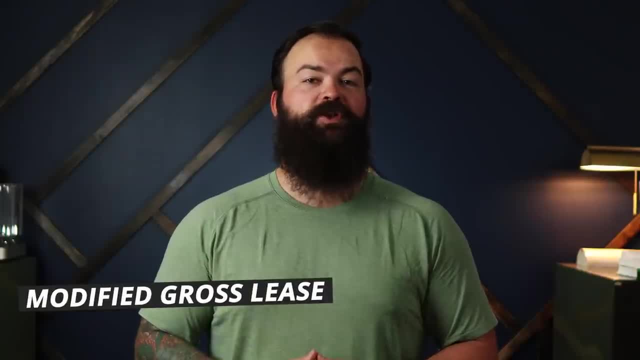 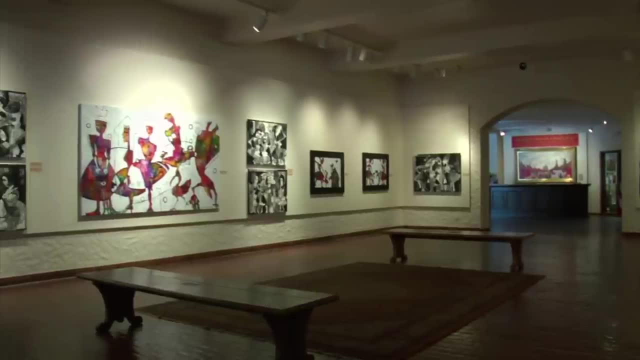 Modified Gross Lease. A modified gross lease, or MG, requires the tenant to pay base rent along with only some of the operating expenses. For example, a group wants to open an art gallery in a space that you have for lease. You know that the electric bill will be pretty high, so you create a modified 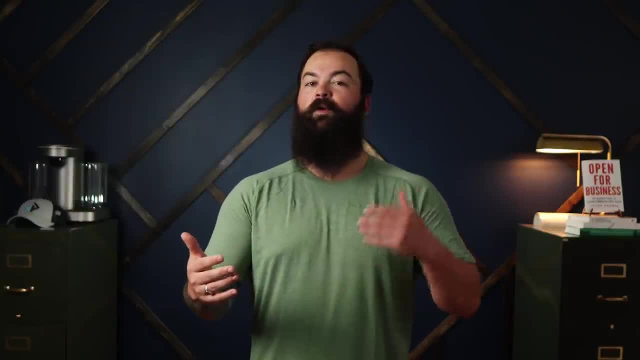 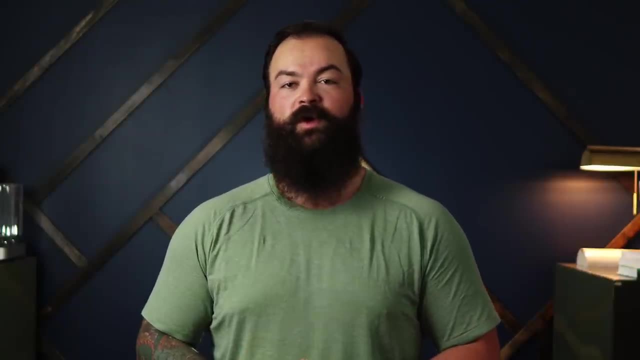 gross lease where the group pays monthly rent along with their electric bill. Calculating the rent for an MG lease is almost the same calculation for finding full-service gross rent. You multiply the price per square foot by the square footage of the space and add this: 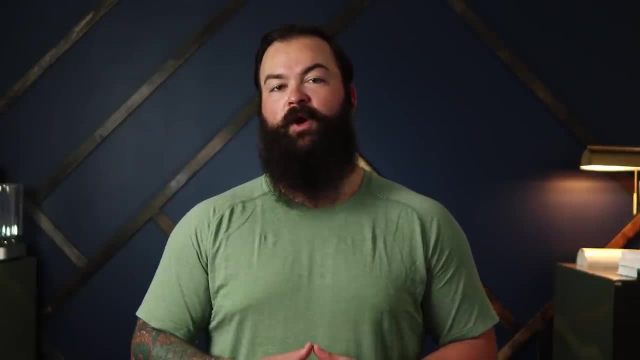 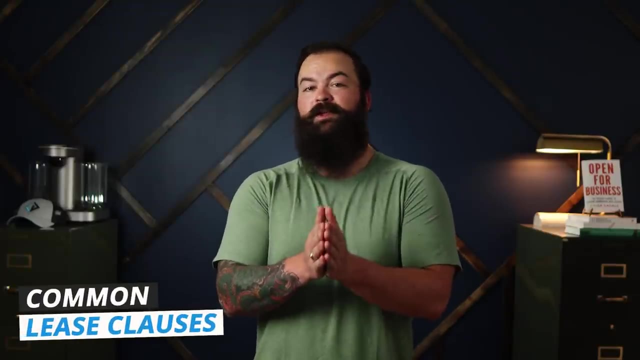 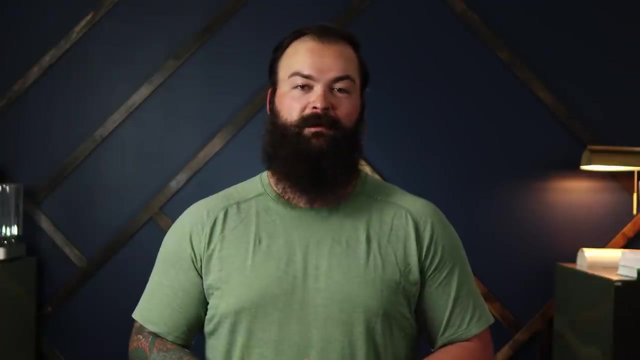 number to the amount of the expense or expenses that you will incur. in addition to rent Lease Clauses, There are a myriad of causes in commercial leases. While it is important that you have your lawyer review your lease, you should also understand the terms on your own as well. Here are a few important clauses to keep in mind. Sub-Lease Clause. Sub-leasing is where a tenant leases unused space in their lease agreement to another tenant. The tenant's lease agreement with the sub-tenant is independent of the lease agreement between the tenant and the landlord, Often referred to as the Right to Sublet Clause. the Sub-Lease Clause states: 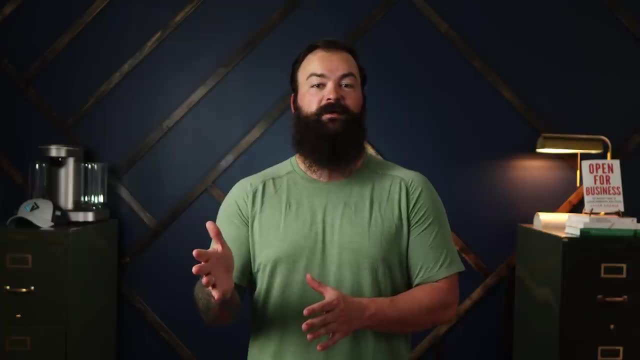 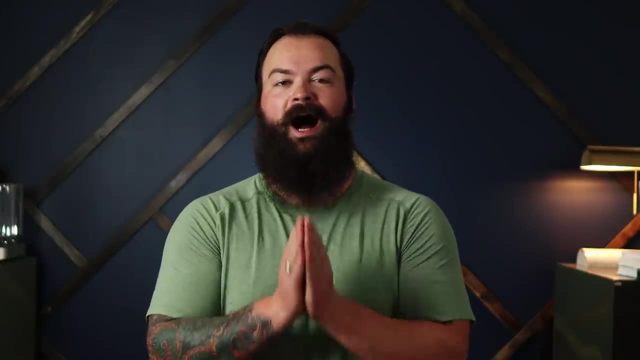 that the tenant does not have permission to lease a portion of the space in their lease agreement to another tenant unless consent is given by the landlord. Now, as always, with all of these commercial real estate terms, I highly recommend you have your attorney review or put together your leases. 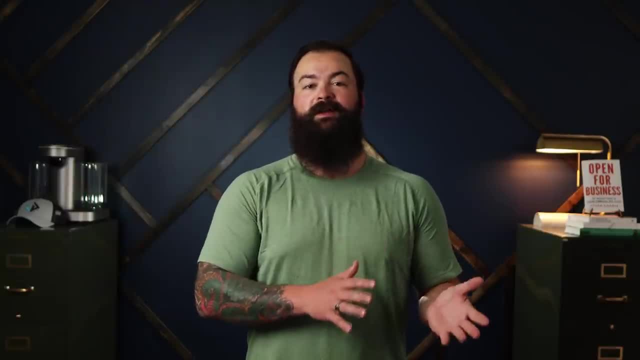 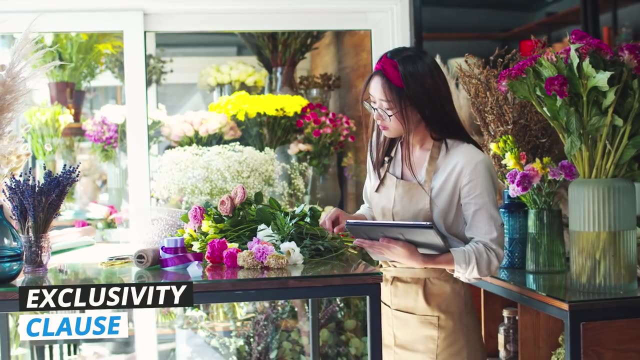 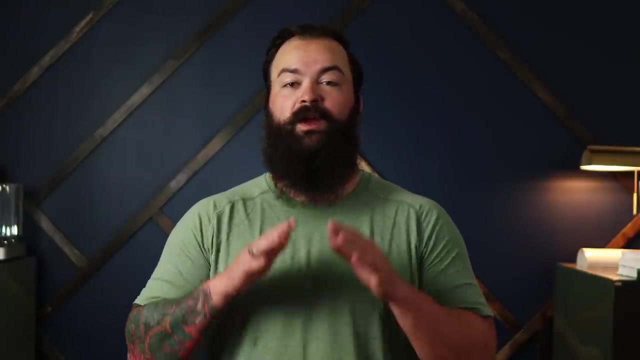 Lease Clause. This clause is important because any additional space that you do not use but is included in your lease could provide you with additional income. Exclusive Right: The Exclusive Right Clause, or Exclusivity Clause, is often found in retail leases, but can be seen in any industry, and it gives the tenant the right to be the 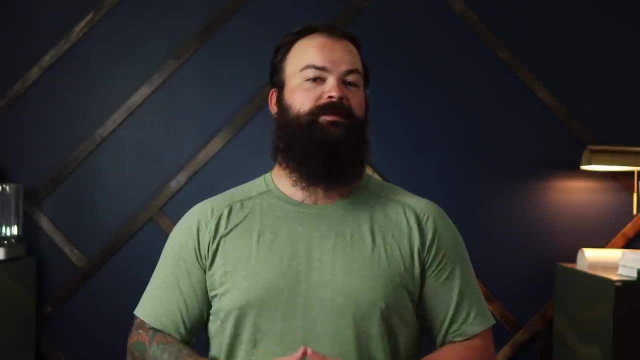 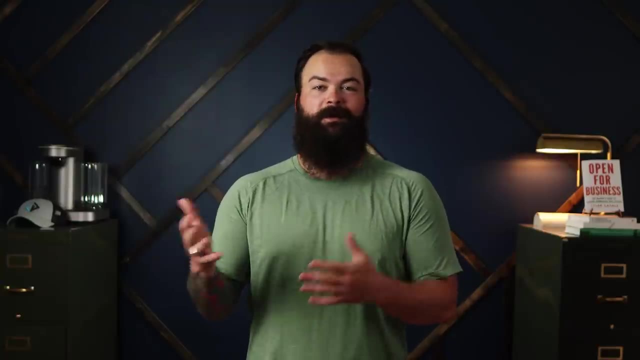 only business that sells a certain product or provides a specific service. For example, if you decide to open a nail salon and a prominent strip mall, you would not want another nail salon to be in that strip mall. Why? Because they are a competing business and have the potential to take some of your customers. So go for that Exclusive Right Clause Now. also, as a landlord, you probably don't want multiple businesses in the same industry within your property because one of them is likely going to go out. So definitely something to keep in mind for the landlords as well. 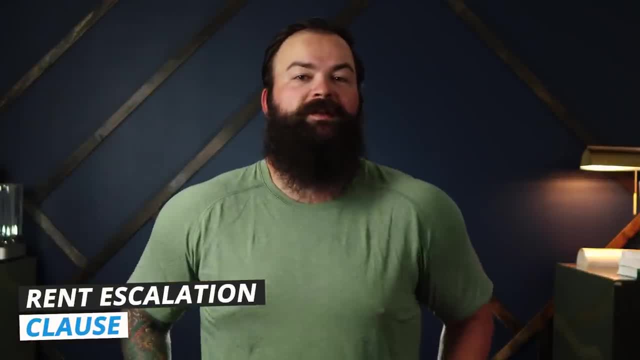 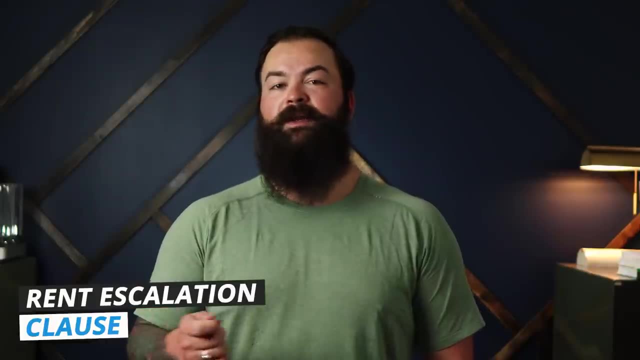 Rent Escalation. When leasing a space, your rent can increase on a yearly basis or during any renewal options. This is what the rent can increase on a yearly basis or during any renewal options. This is what the rent escalation clause covers. A rent escalation clause explains how much of an increase in rent a tenant will be subject to. For example, a landlord may state that there will be a 2% annual increase in rent, or a landlord may state that the rent will increase by 5% every two years. Every lease is different. The rent escalation clause is one of the most important clauses because in the long run, an annual 2% increase can greatly affect the overall cost of tenancy. Delivery Conditions: Commercial spaces can be delivered in a variety of different conditions. Sometimes you may lease a space that is basically move-in ready, and sometimes you may lease a space that is nothing more than a skeleton of the building. 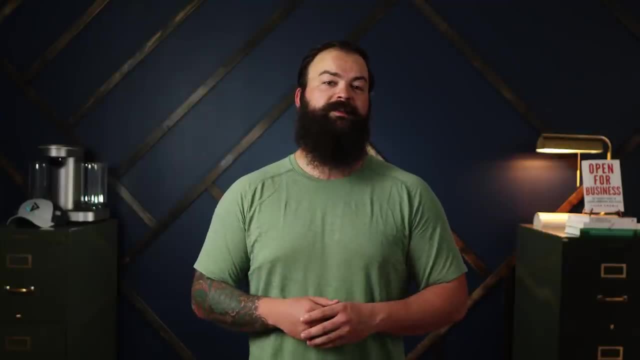 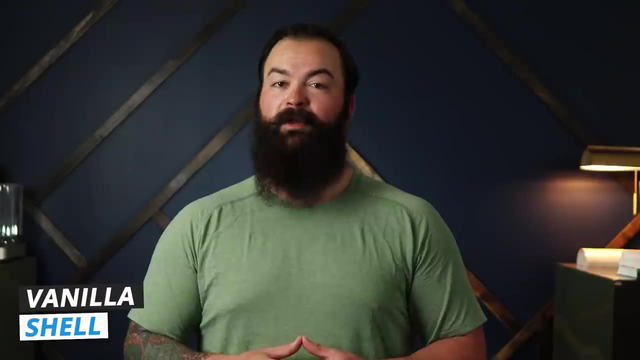 Let's dive into a few of the most common delivery conditions for commercial leases. Vanilla Shell: A vanilla shell lease, or white box, can be one of the sweetest deals you get as a tenant. Build-out costs for vanilla leases are what makes them so desirable. You spend the least amount. 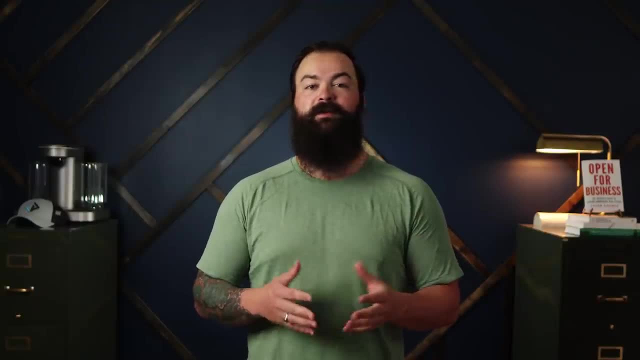 if any, as a tenant during the build-out of a vanilla shell lease. compared to any other delivery condition, Your costs for build-out mostly reflect the cost of your tenant-specific amenities, and this condition is good for landlords because it also helps you lease the spaces faster. 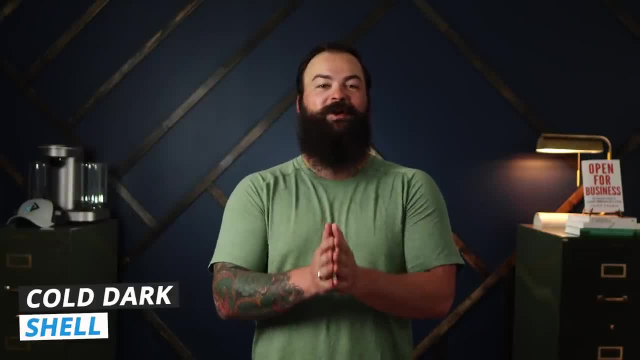 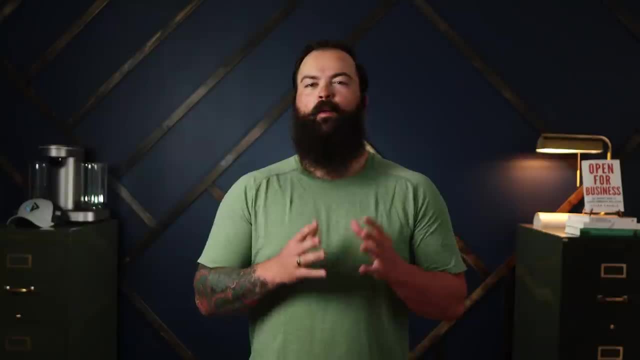 Cold Dark Shell. I know this name is very creative, but cold dark shells are exactly what they sound like. You can expect the spaces to be down to the studs of the building. It's essentially a skeleton. Now why would you want a cold dark shell lease? Aren't the build-out costs going to be high? 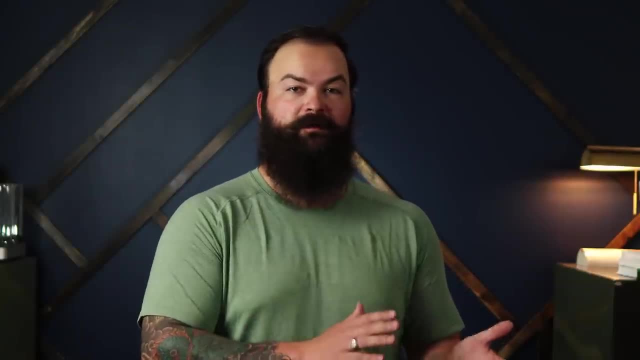 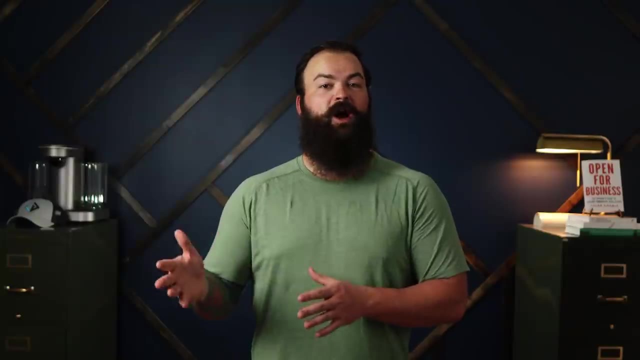 Well, yes, cold, dark shell build-out costs are higher than any other delivery conditions For the tenants. they're obviously cheaper for the landlords, but there is an incentive. Landlords generally offer a lower rent and a higher tenant improvement allowance since the build-out costs will be high for the tenants. As a landlord, that can be pretty attractive when you're finding tenants because it's more affordable on a monthly basis and, with the incoming tenants spending so much money on the space, you know that they're committed to staying there for at least a while. 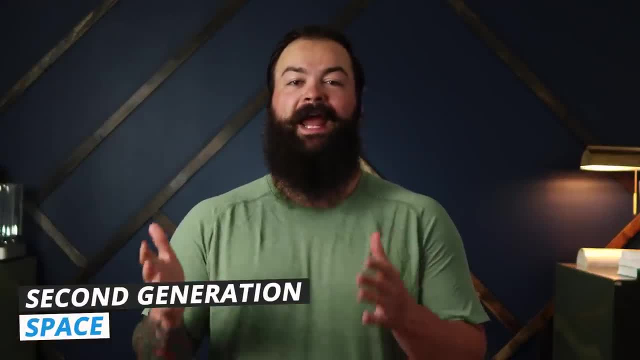 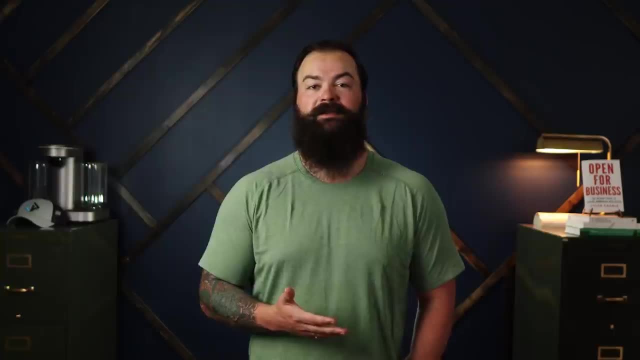 Second Generation Space. Second generation spaces are the hand-me-downs of commercial real estate. Now, what makes them so attractive is that it could require little to no build-out costs, depending on the previous business and tenant. If you're looking to open a restaurant, 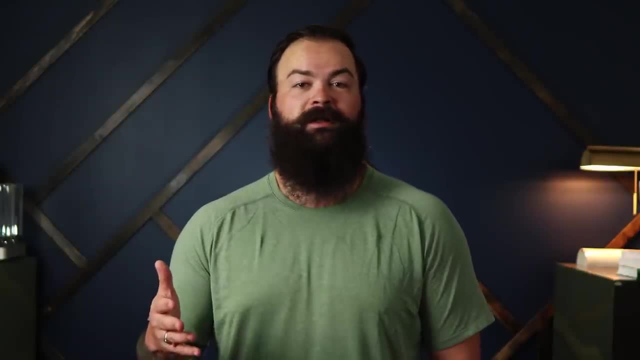 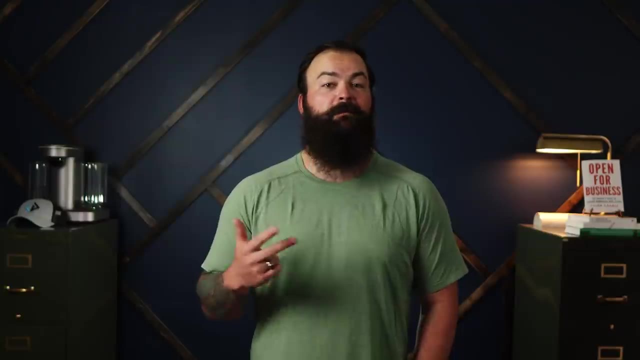 a second generation space where the previous tenant was a restaurant may be ideal for you. Why? Because this space is likely to be outfitted with the proper ventilation system, grease traps and more that you'll need in a kitchen. You may find that the lease includes commercial stoves, refrigerators, walk-ins. 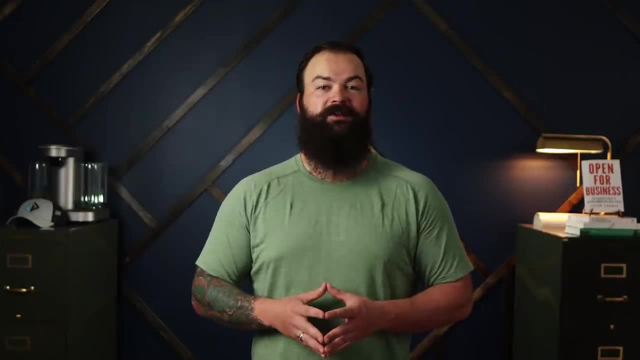 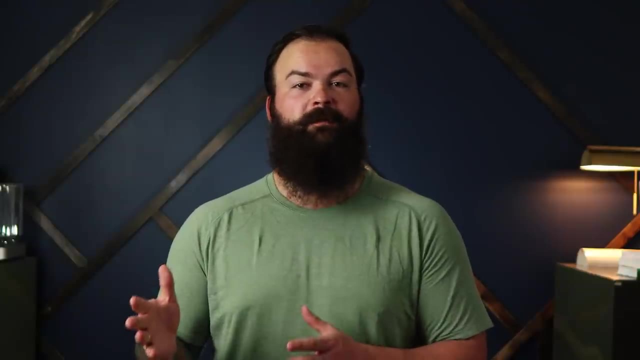 any number of items. It's not uncommon for the new tenant of a second generation space to slap some paint on the walls, lay new flooring and open for business. As a landlord, you'll definitely want to target businesses that could take over these second generation spaces a lot faster than any other tenant, because you want to make sure you keep that vacancy low. Now, one downside of a second generation lease is that it's going to reflect the previous tenant Also if this space was previously leased to a long-term tenant. 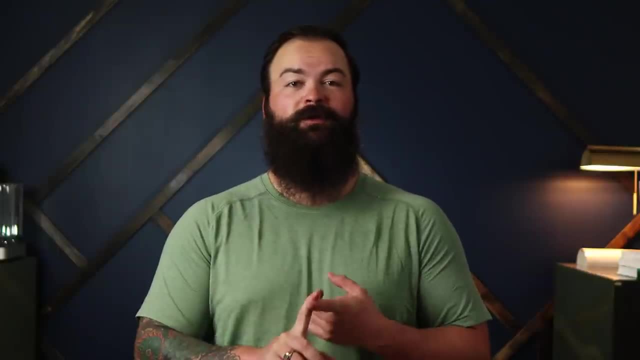 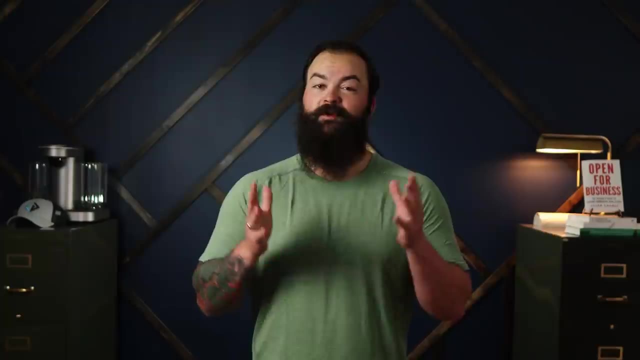 you may need to make sure the space is up to date. So by now you know a few general commercial real estate terms and the common delivery conditions of commercial spaces, But there's still a ton to learn, especially if you're a first-time commercial real estate. 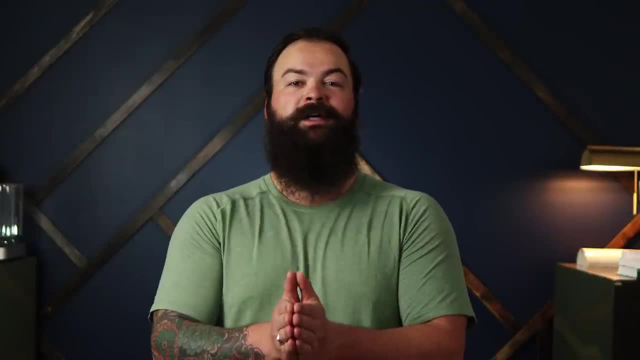 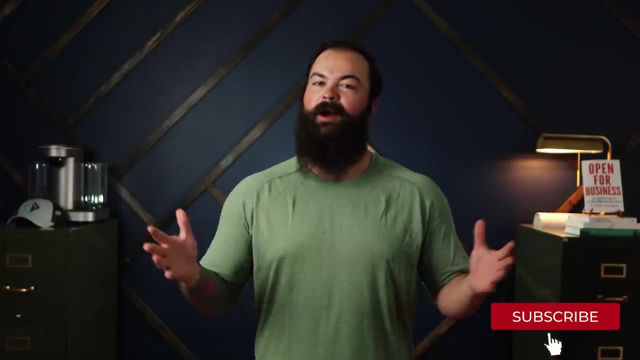 investor. I hope this overview provided you with some helpful information. Let me know in the comments what terms you'd like to know more about, And if you're interested in learning more, hit that like button. subscribe to BiggerPockets and stay tuned for more commercial real estate videos. I'll see you next time on BiggerPockets. 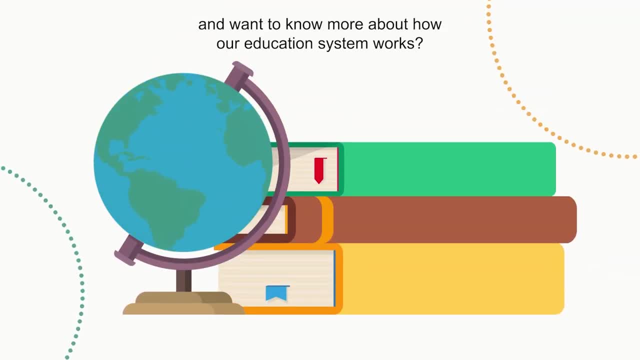 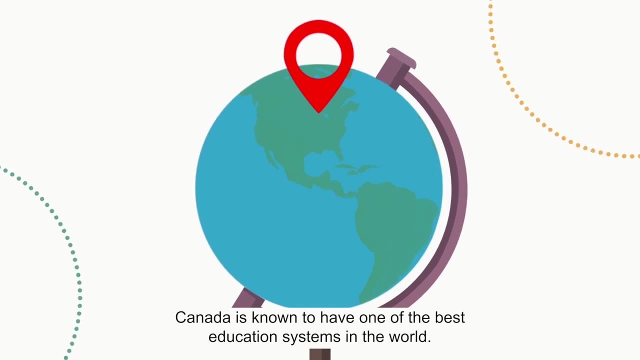 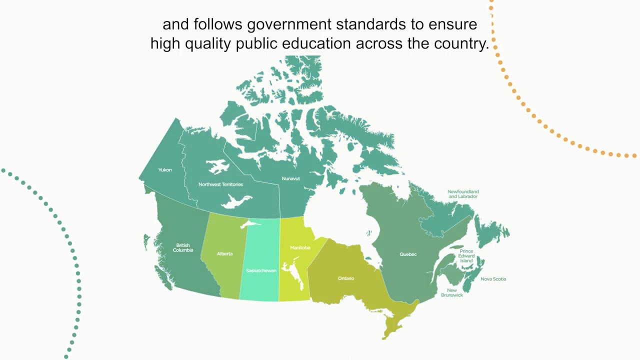 Are you interested in studying in Canada and want to know more about how our education system works? Canada is known to have one of the best education systems in the world. Each of Canada's 13 provinces and territories runs their own school system and follows government standards to ensure high-quality public education across the country.